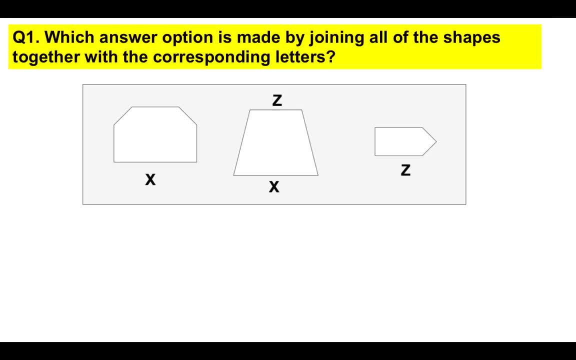 of the Shaggy's. Okay, so the answer is A, B, C, D or E. So what we have to do is look at the shapes in the rectangle above the shaded rectangle and we have to join the letters together where. 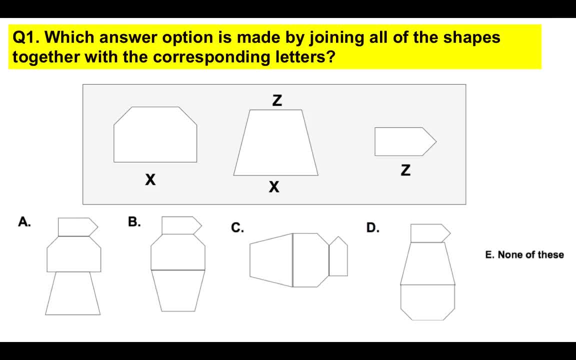 they correspond to decide which of the shapes from A, B, C or D it is, or if it's none of them, we would select E. So if we take X and join that with that part there, then that would look like that. 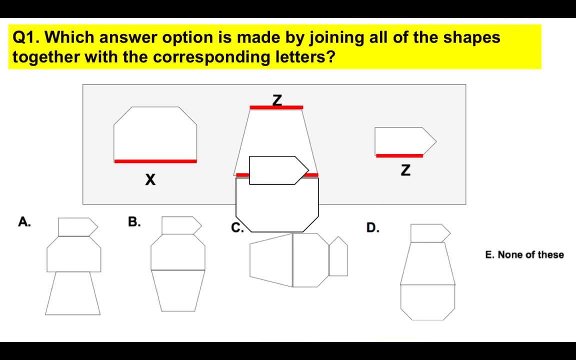 Then if we take Z, put Z together there at the top and then put that shape there, then the only option it could be is, of course, D, It's certainly not A, it's not B, it's not C and it isn't E, none of these. So the correct answer to question number one: 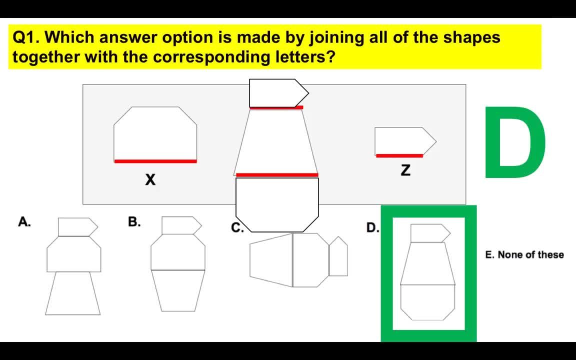 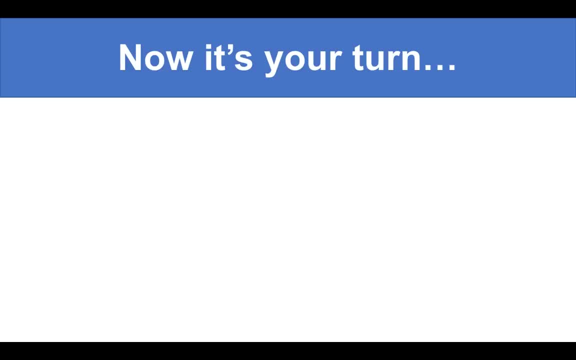 is D, and this is a common kind of spatial reasoning test question where you can get off the ground running quickly and get your marks going. So have a go at this one. Put your answer to spatial reasoning test question number two in the comments section below. 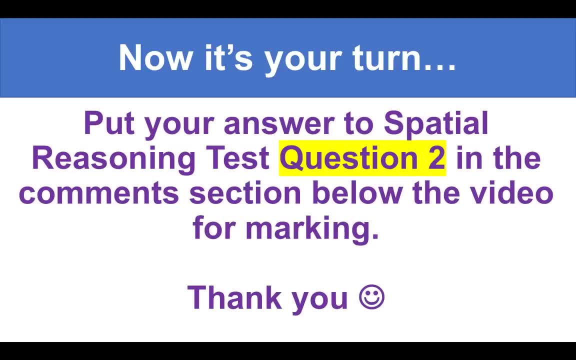 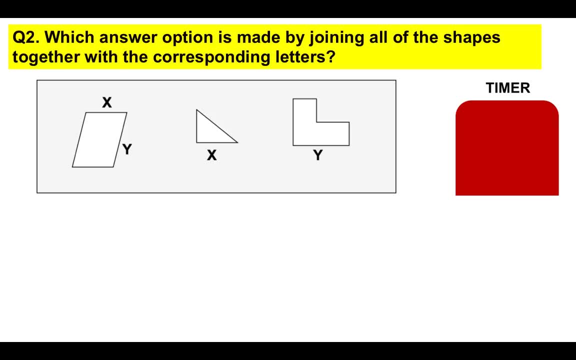 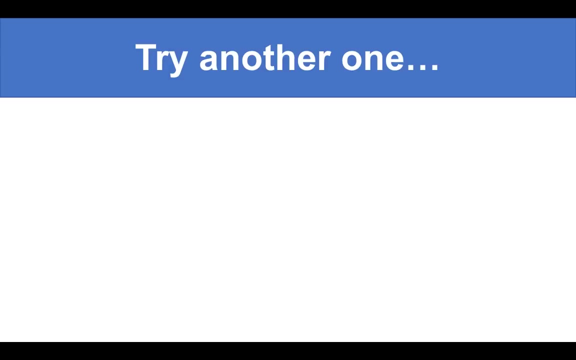 and I'll see you in the next one. Subtitles by the Amaraorg community. Okay, well done. So hopefully you got that correct. Don't forget to put your answer in the comments section below. Have another go at one similar, because I want you to get. 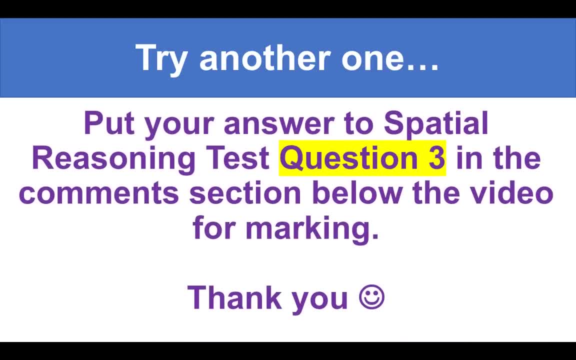 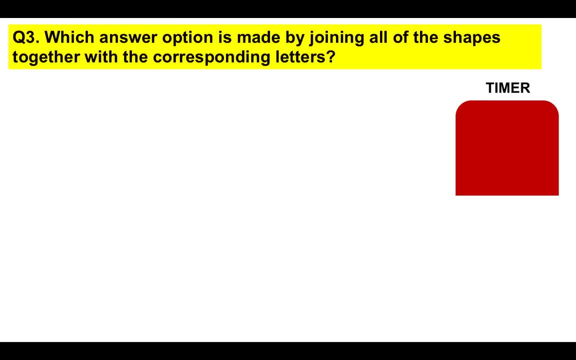 used to these basic type of spatial reasoning test questions. Put your answer to question three in the comments section below for marking. Here we go. So which answer option is made by joining all of the shapes together with the corresponding letters A little bit tough. 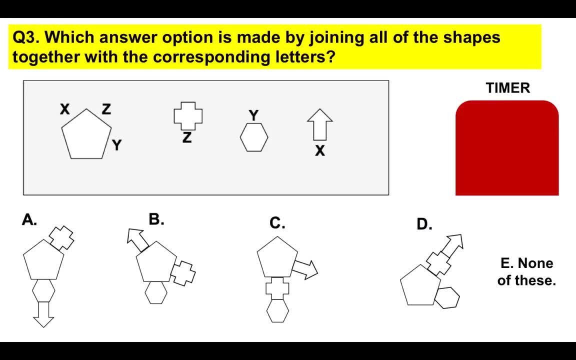 for this one, so you'll have to work a bit quicker. Is it M, B, C or D? Is it A, B, C, D or E? None of these, And here's your timer. Okay, brilliant, So well done If. 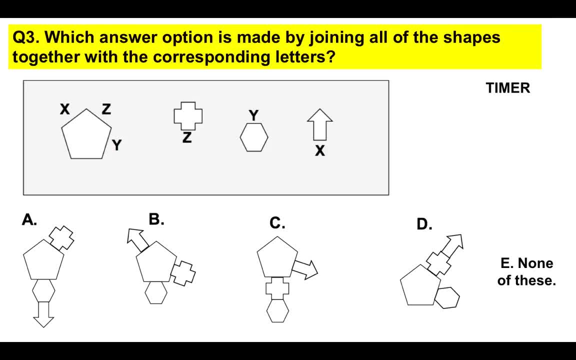 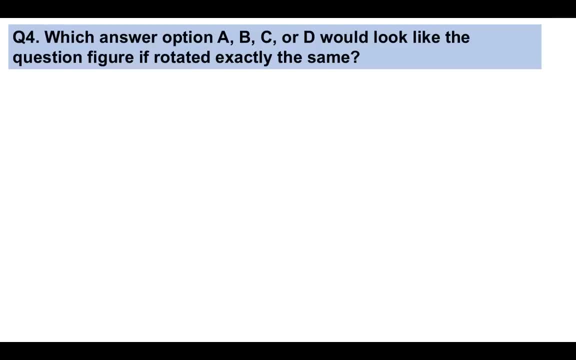 you're finding that the timer is going too quick and I am putting you under a bit of pressure here. please feel free to pause the video, because I would rather you got these correct. Okay, question number four. Let's change the kind of spatial reasoning test. 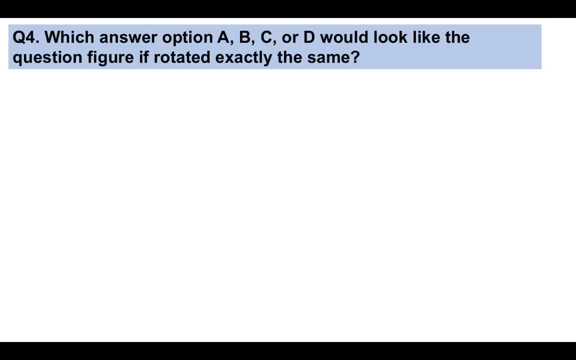 type question Which answer option A, B, C or D would look like the question figure if rotated exactly the same. So this is the question figure and what we have to do is rotate it to the left or anticlockwise through 90 degrees and work out which one it would be: A, B, C or. 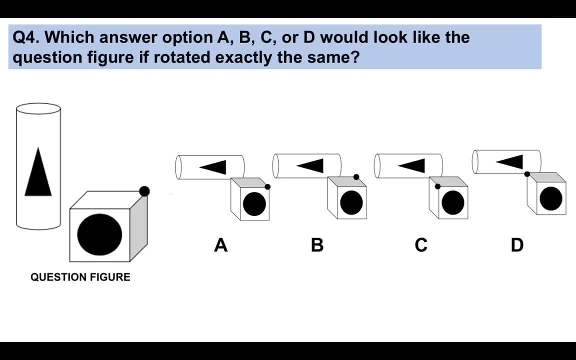 D. Now, on initial inspection they all look the same, but they're not, And what we have to do to answer this is to pick one or two parts of the question figure shape. So what we would do here is we would pick one or two parts of the question figure shape and we 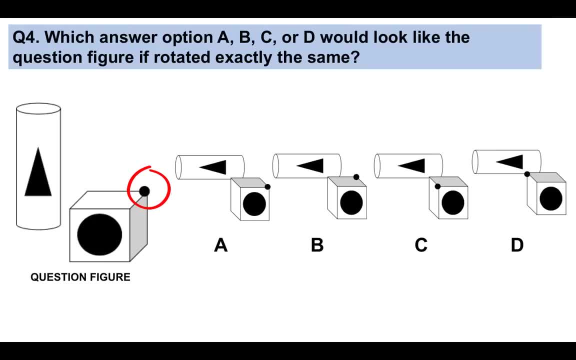 would pick that small black dot or circle And we would also focus on the shaded part. Okay, that shaded part. You only have to focus on the two parts. Don't look at it as a whole And then go through A, B, C or D, rotate it 90 degrees in your mind and go through. 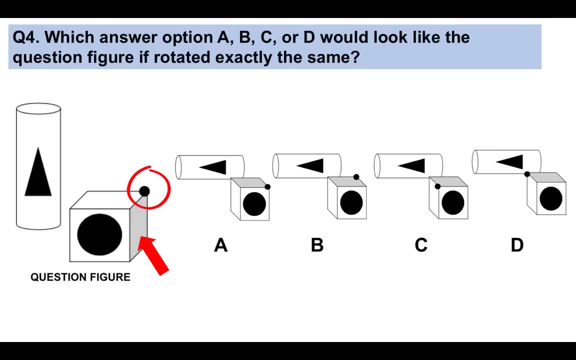 a process of elimination until you get the correct one. So it simply can't be A, because if you look at that black dot, it's actually there on the top right-hand side and it actually forms at the back on the question figure. 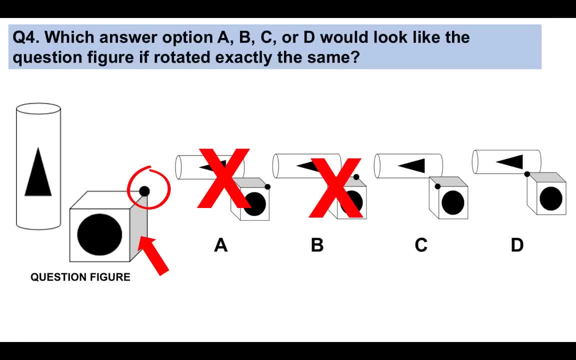 So it's not A. If we look at B, well, yes, the black dot there is in the correct position. However, you look at the shaded part, it's in the correct position, but the black dot has stayed exactly where it is and it needs to rotate, So it's not B. Then, if we look 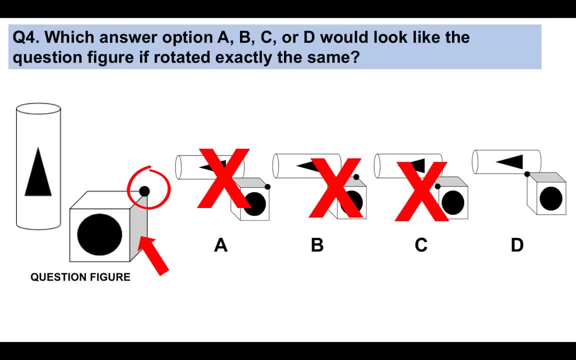 at C. it can't be C because, even though the shaded part is where it should be, the black dot is not. Therefore, the correct answer is D to question four. Okay, now it's your turn. Please put your answer to Spatial Reasoning Test, question number five, in the comments. 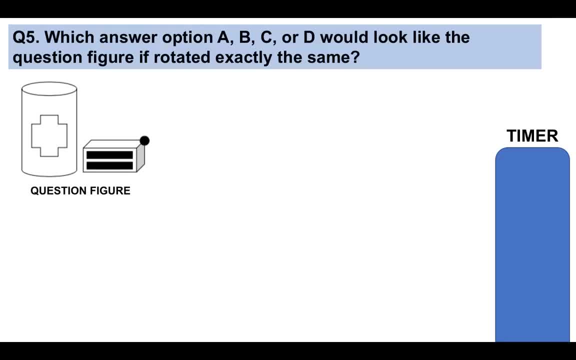 section below for marking, and we have a timer as well. So question Which answer? option A, B, C or D would look like the question figure in the top left if rotated exactly the same. Here's your timer. Okay, Hopefully. well done, You've done a good job at drawing. 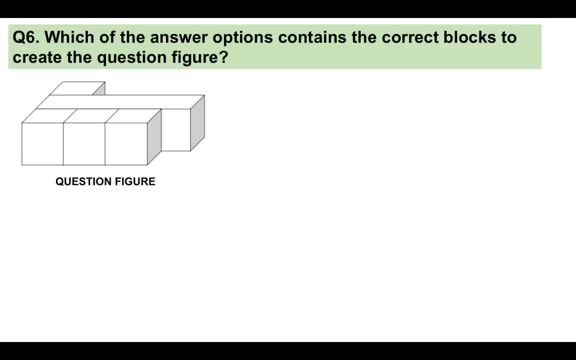 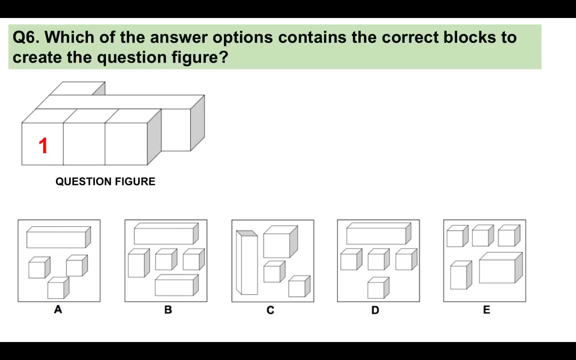 got that question correct. Question number six: Let's look at a different kind of spatial reasoning test question. Which of the answer options contains the correct blocks? to create that question figure We have to look from A, B, C, D or E. The way to do this is to: 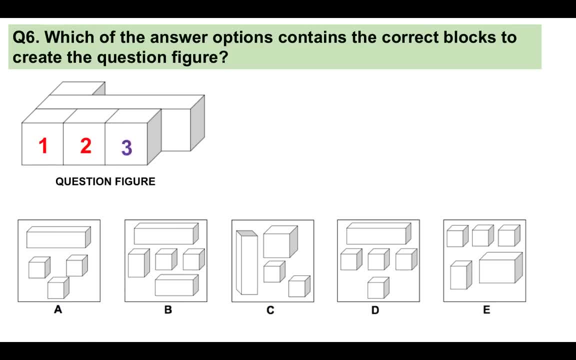 calculate or to add up how many small blocks there are first of all, and you'll see that there are four. Then there's also one large rectangle block. We are, from the answer options, looking for four small square blocks and one large rectangle block. If we go through, 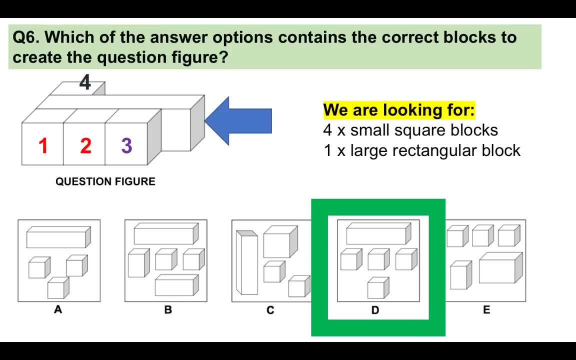 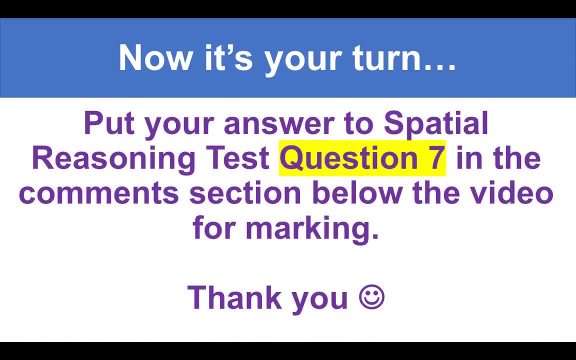 a quick process of elimination. we will see. the only answer it can be is D. Now it's your turn again. Please put your answer to spatial reasoning test question number seven, in the comments section below the video for marking. Here we go. There's your timer. Which of the 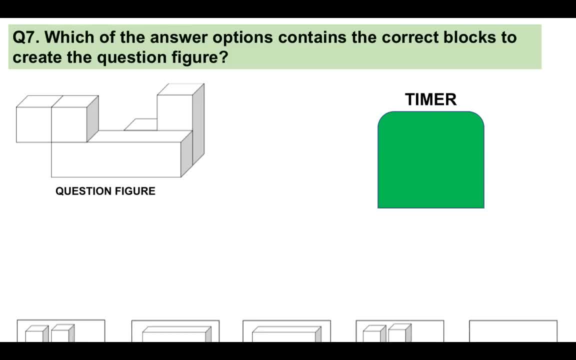 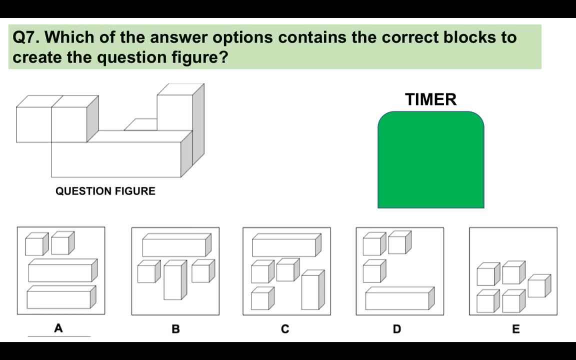 answer options contain the correct blocks to create the question figure below A, B, C, D or E. You have the time. It takes the time. You have the timer to go down to get the correct answer. Here you go. Okay, well done, Let's. 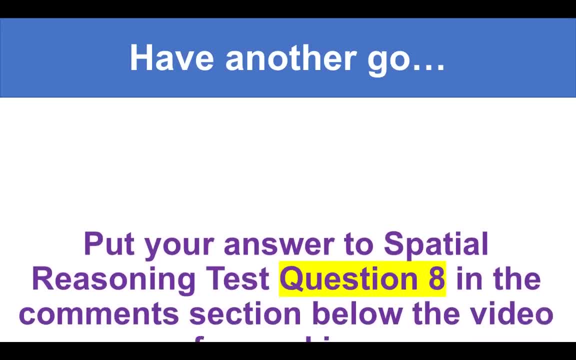 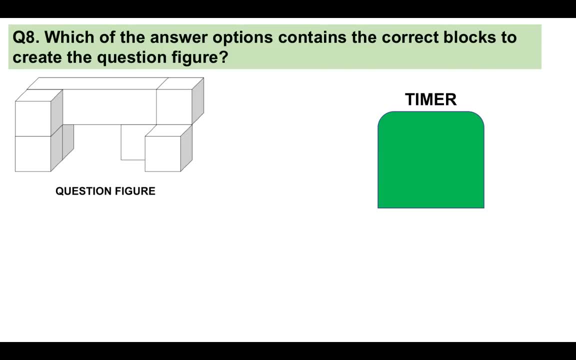 move on now to question number eight. I want you to have another go at a similar question like that. Again, put your answer to question eight in the comments section below the video for marking. Here you go. Which of the answer options contains the correct blocks to create. 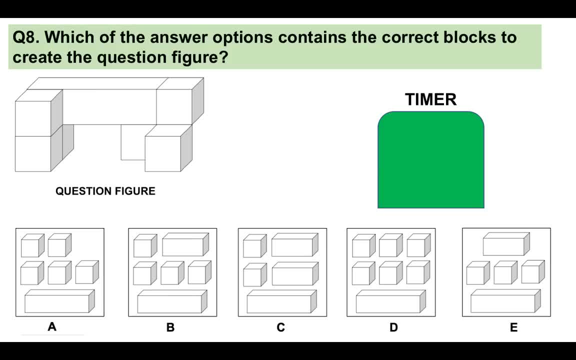 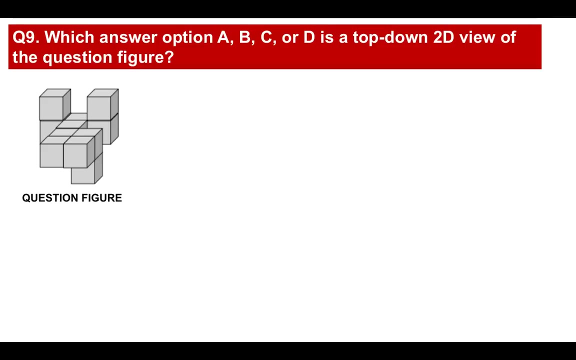 that question figure right there. Is it A, B, C, D or E? Be careful with this one. It's not that easy. Here you go. Okay, fantastic, You're doing really well. Let's make it a little bit tougher. now. Question number nine: Which answer option? 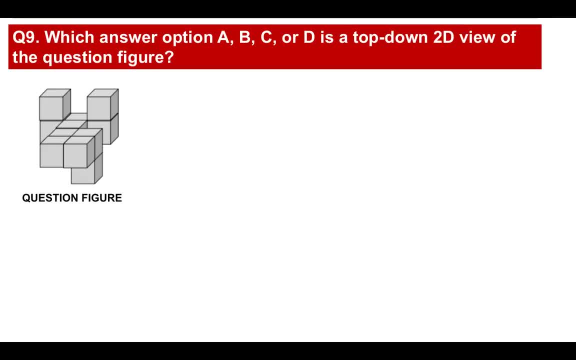 A, B, C or D is a top-down 2D view of that question figure. Okay, If we were looking down on the question figure, is it A, B, C or D? Slightly tougher because you have to visualize looking down on the. 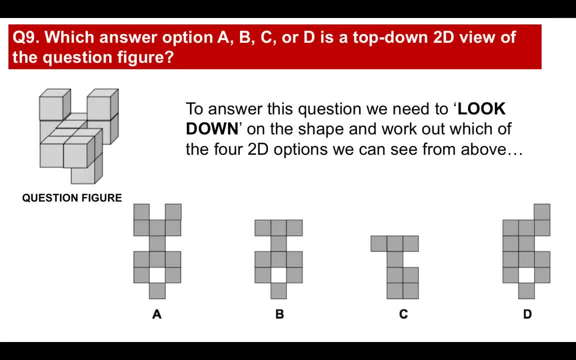 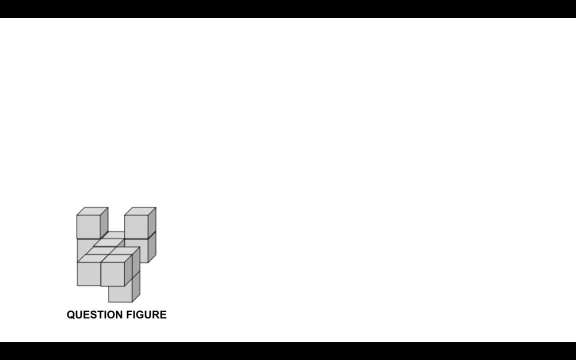 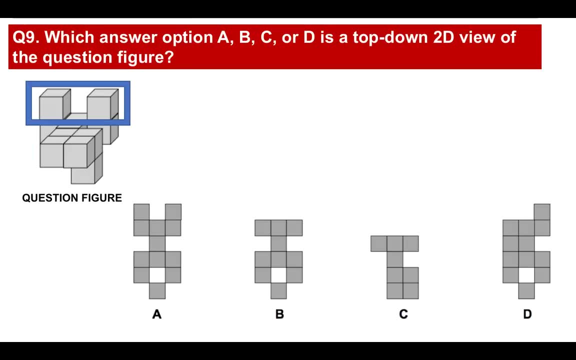 figure To answer the question. we need to look down on the shape from the top and work out which of those four options we can see from above. If we just take out the question figure and think about looking down from above and go back to it, we could see there across. 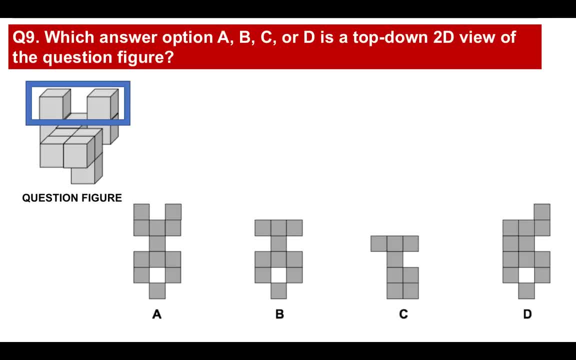 the top that even though those two square blocks left and right are protruding, if we look down it would actually look like three running across. It can't be A because there's only two there across the top and it can't be D because there's only one there across. 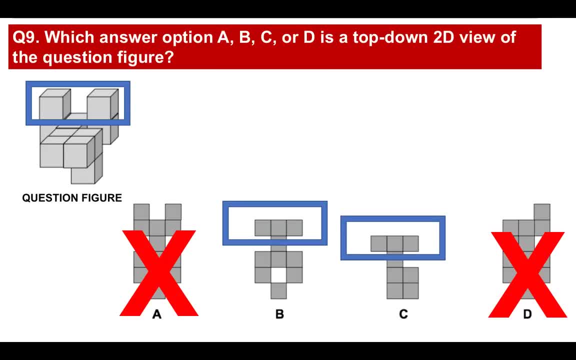 the top. Therefore, it can only be either B or C. You'll get really good at these when you practice them, because you just work through a process of elimination. It's either B or C, Then what we would do is put a line across the center there and think: well, there has. 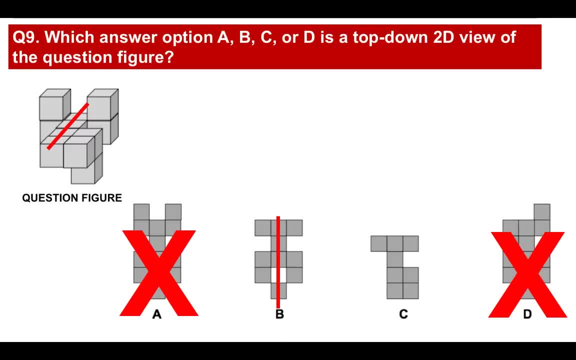 to be four squares with no gaps across the middle. Well, it can't be that one, because there are four, but there's a gap on the fourth one, So the only correct answer it can be is C. Okay, Now it's your turn. Put your answer to spatial reasoning test, question number 10. 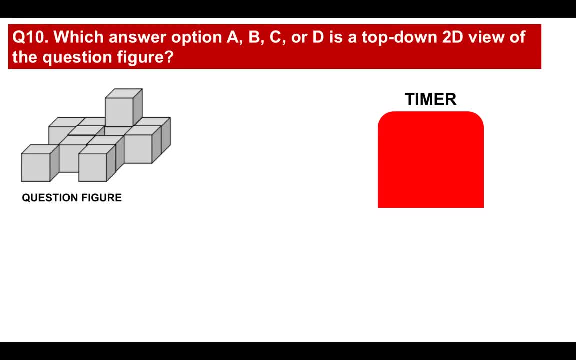 in the comments section below the video for marking. Here we go. Which answer? option A, B, C or D is a top-down 2D view of that question figure right there. It's quite difficult. Okay, Here's the timer. Off you go. 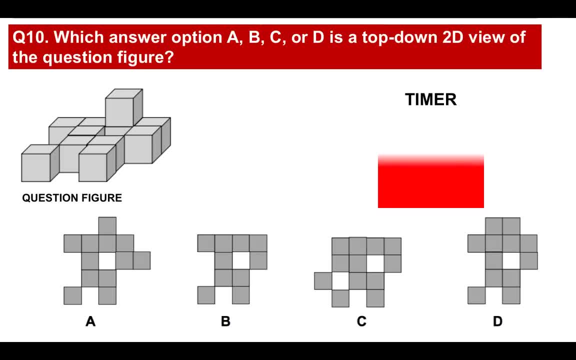 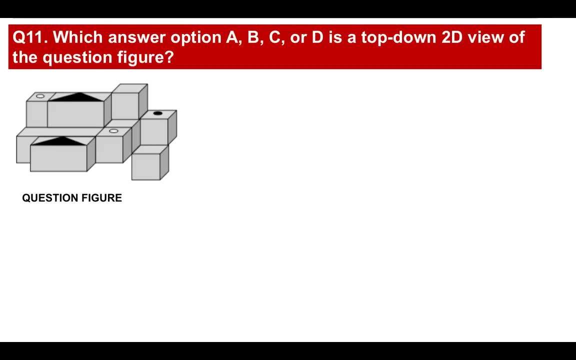 Excellent, Well done. Okay, Let's move on now to question 11.. This one is even harder and I'll give you a go at one of these in a second. Which answer option again A, B, C or D- is a top-down 2D view of that question figure. Is it A, B, C or D? Now, when you 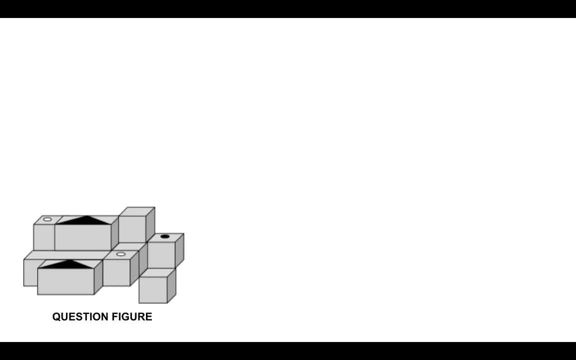 look down on that figure, it looks quite confusing. but all you have to do is pick the answer and pick one particular part of it to get the answer. So if I draw a line there from the white circle across that black triangle and down across and then think what would? 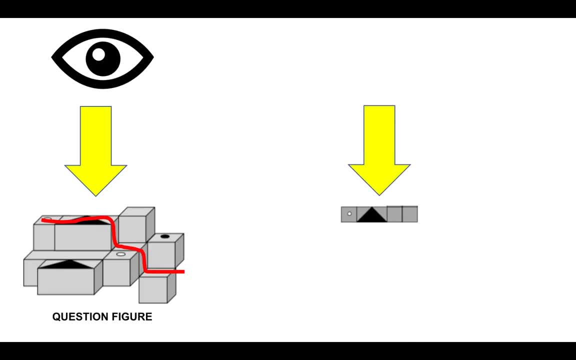 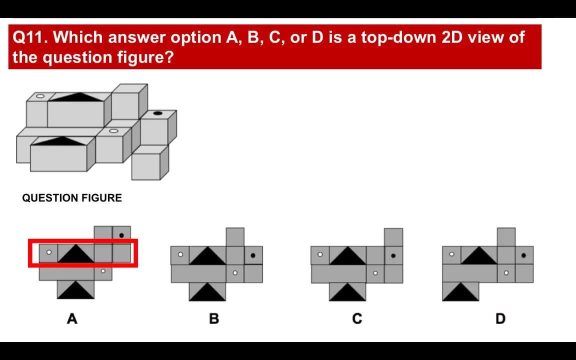 that look like Looking down, it would look like that. Then all I need to do is have a look at the options, and I can see there is only one of them that has that shape in it. Therefore, I don't have to do any other work, because I know that is the correct answer. 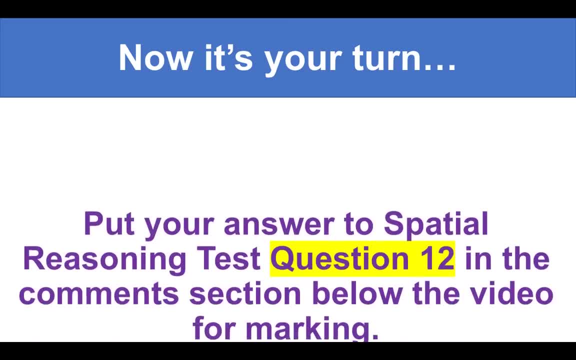 and A is your correct answer. Okay, Have a go at question 11, B, C, D, C or D. Okay, Have a go at question 11.. Have a go at this one. It's quite tough. this one Put your answer to spatial reasoning.